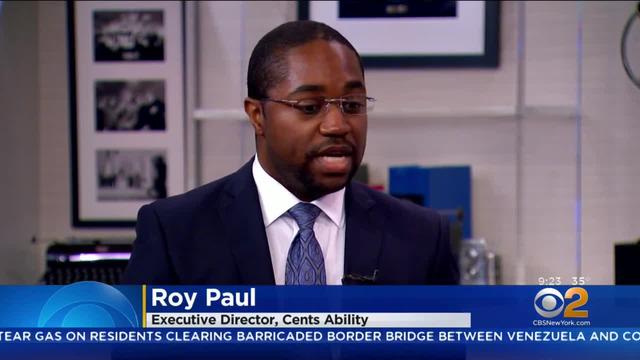 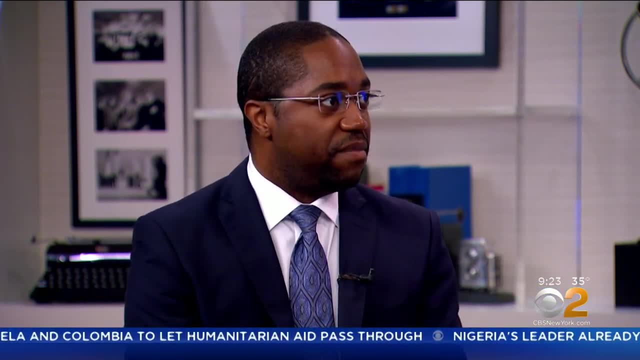 Look, we're in Harvard Business School, We have access to resources, yet we are struggling with personal finances. And so they said, in that midst of all the chaos, let's do something to give back. And that's when Sensibility was founded. And a lot of kids, as teenagers, are starting to get their first jobs. What advice do you have for them in terms of jump-starting their savings? Yeah Well, if you look at the picture more broadly, it's very, It's very stark, right. You've got over half of Americans- 57%- that have less than $1,000 in their savings account. 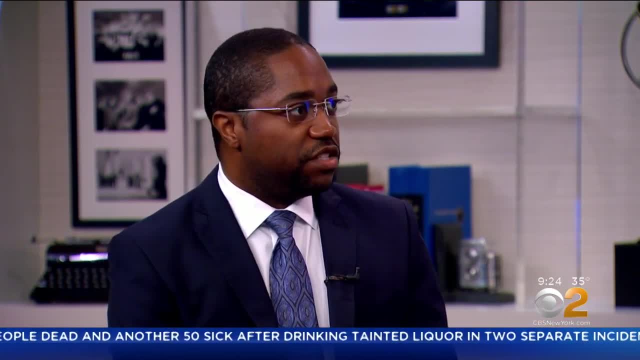 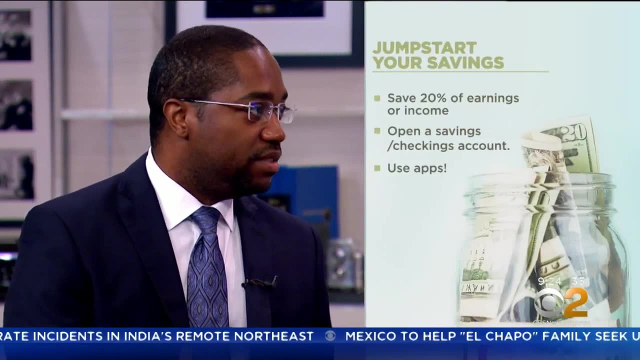 These are Americans, right, And so when you look at teenagers, it's a perfect opportunity to teach them at a very early age how to save. So the 20% rule is very simplistic for us. We like to tell our young people to follow it. 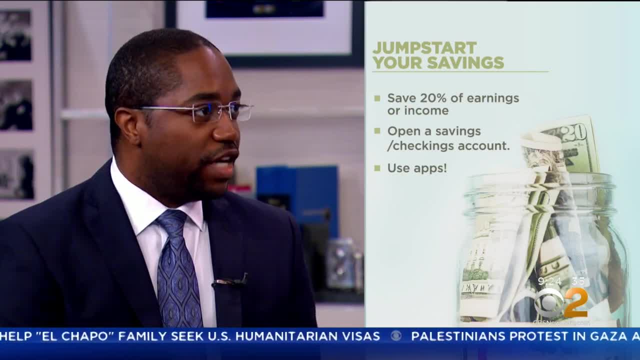 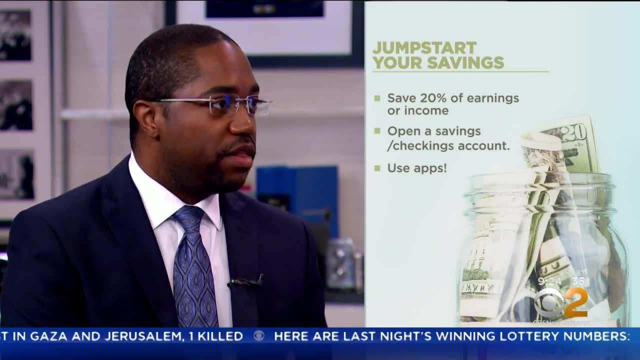 Whenever you get money, take 20% and save it right, Don't touch it. And so kids say: you know, what can I differentiate from? And we say: don't differentiate Whenever you get money, whether it's from graduation fees. 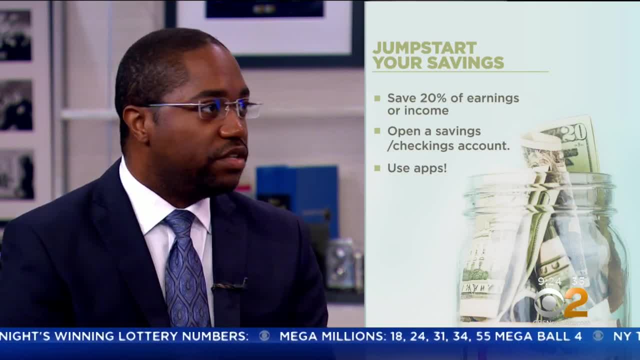 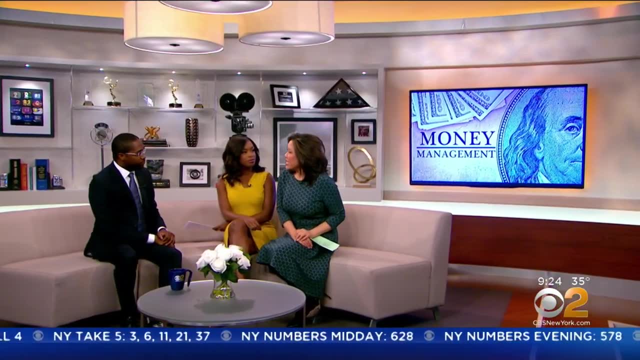 You mow the lawns. you have three jobs. you work part-time at McDonald's. get into the habit of saving 20% of whatever you earn. That's such a great idea, And I guess an easy way to save it is to have an account at the bank. 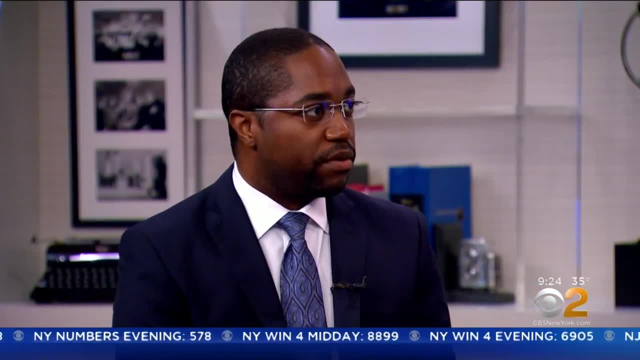 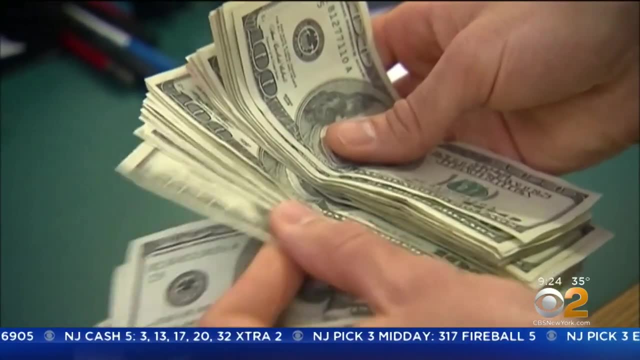 Yeah, that would be preferable. We have a lot of young people who go through our program who come from lower-moderate-income communities and their idea of a financial institution is a check-cashing place, right, And they get gouged with fees left and right. 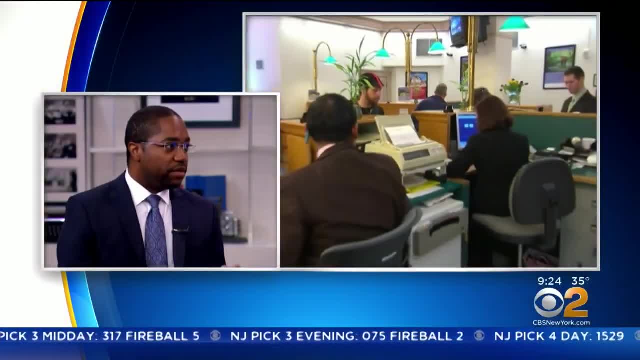 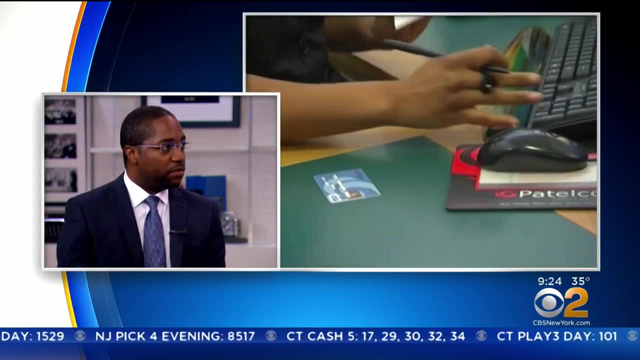 And so we say to them, especially to parents: you know, when I was younger, my mother would take me with her when she went to vote, and that was a very memorable experience. And similarly, when I started earning money, she took me to the bank and she said: you're going to open up a savings account. 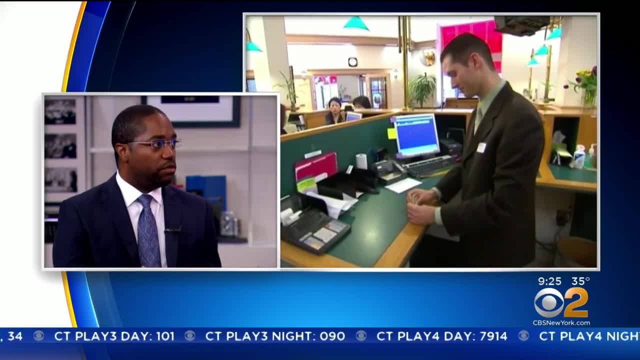 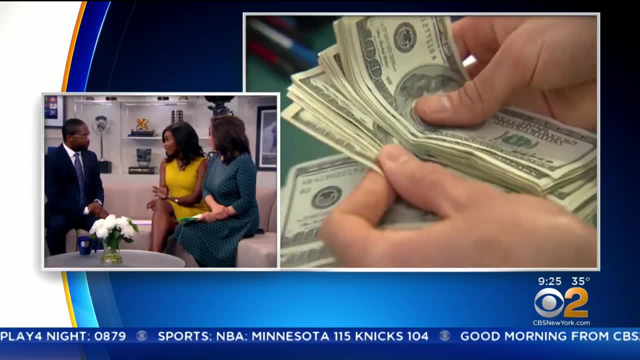 You know, learning to develop trust in a financial institution that will safeguard your finances is the best thing to do, And so I say, take your kids to open up an account. And this day and age, you know, especially with technology, there's a lot of apps that are available that can sort of help you track your finances. Any that you suggest that would be useful to teens? Sure, Well, I use Mint and it's a perfect one. It aggregates all of your accounts and it helps jumpstart your savings. So you can say: I want to put 20% automatically into this account. 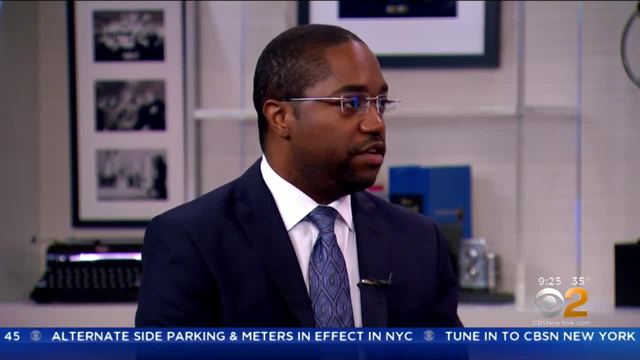 You can download your credit card statements. Everything is in one place. If you don't know your FICO score, it's there. As soon as you open up your app, it's right at the top, Because I talk to people all the time- friends of mine. 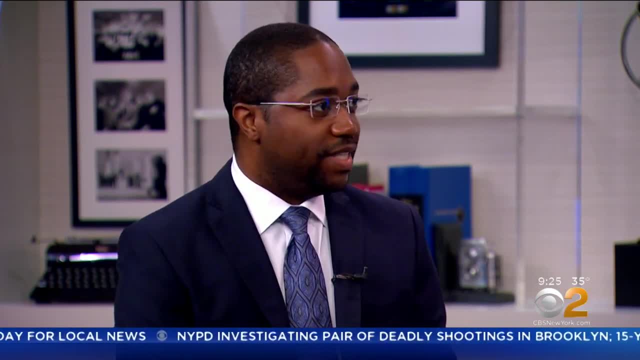 They're in their 30s- 40s, They make great money And I say: what's your credit score? They have no idea, right, And so it's a perfect way to do it. If you can download Uber, you can download some of these apps to help you save.